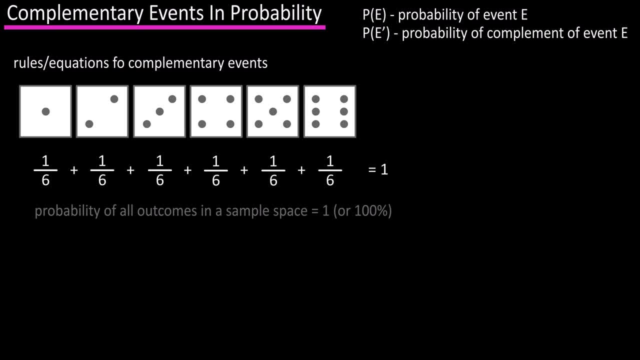 one over six and if we add them up we get one. So the probability of all outcomes in the sample space equals one or 100 percent. With that knowledge, the probability of event E plus the probability of E prime equals one. For instance, in our example rolling a one or a two in a die. 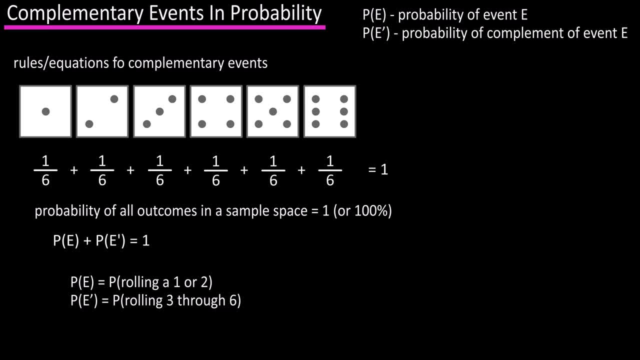 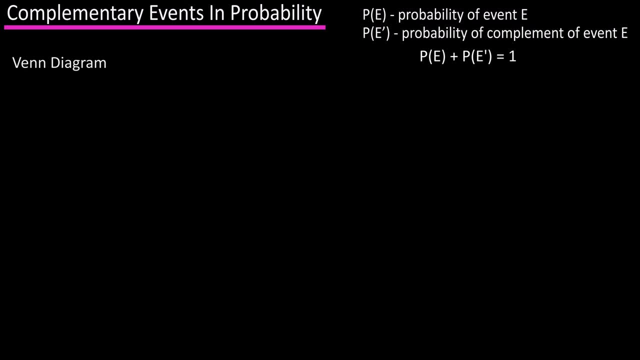 would be the probability of event E, and rolling a three through a six would be the probability of E prime. If we add probability of E and E prime, we get one. To see this visually, we can look at a Venn diagram. So here is a square. 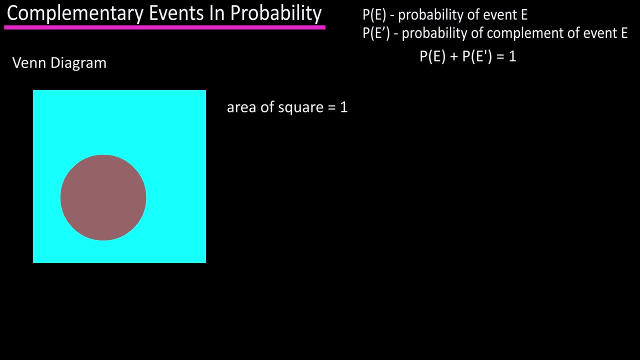 and the area inside this square equals one. If we put a circle in this area and let the circle represent the probability of E, then the area outside of the circle represents the probability of E prime. So if I said the area of E is 0.35, then one minus 0.35 equals 0.65, and that is the 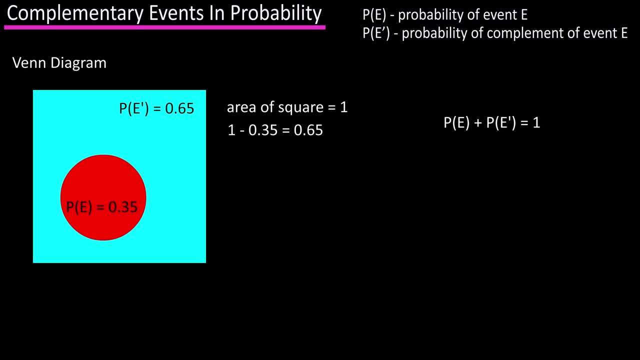 area of E prime. And, as you just saw, we can use this equation two other ways. First, we can subtract the probability of E prime from both sides to get the probability of E equals one minus the probability of E prime. Or again from our original equation we can subtract the 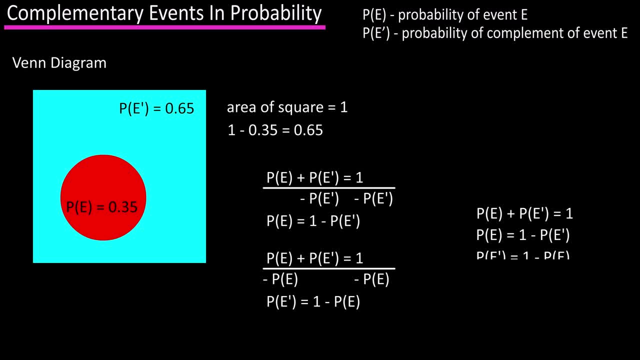 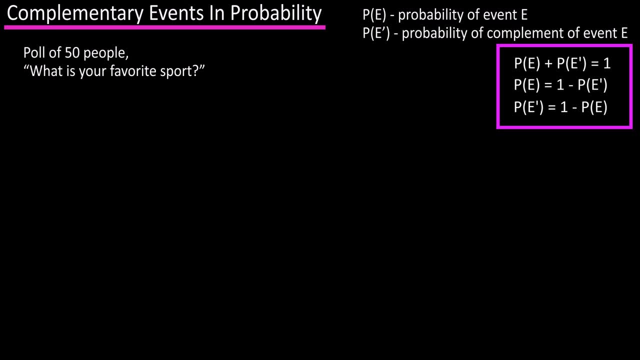 probability of E from both sides to get the probability of E prime equals one minus the probability of E, And these equations can come in handy. For instance, let's say you polled 50 people and asked them what their favorite sport is Using a frequency table. 29 said football. 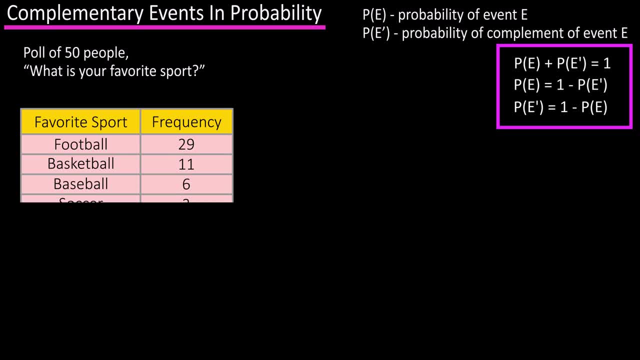 11 said basketball, 6 said baseball, 3 said soccer and one said tennis. Based on the data in this table, what is the probability of randomly selecting someone whose favorite sport is not football? So to answer this, we can use the 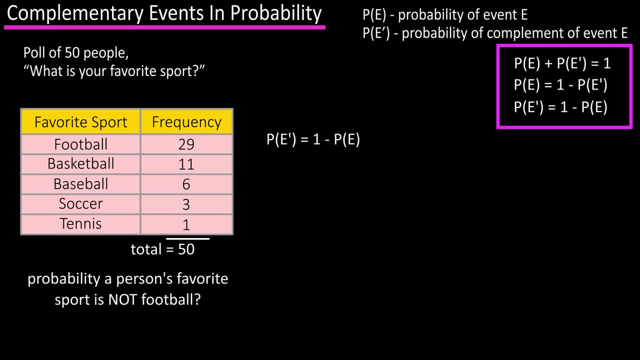 equation of probability of E prime equals 1 minus the probability of E. In this equation, the event E is the probability that football is a person's favorite sport, which is 29 over 50, and E prime is the probability football is not a person's favorite sport. So the probability of E prime. 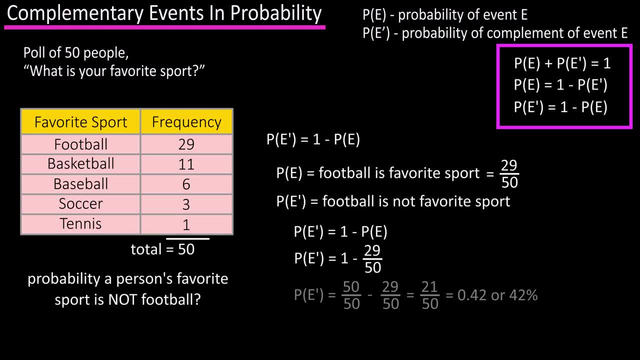 equals 1 minus 29 over 50. Doing some math, we get 50 over 50 minus 29 over 50,, which equals 21 over 50, which equals 0.42, or a 42% probability of selecting someone whose favorite sport is not.